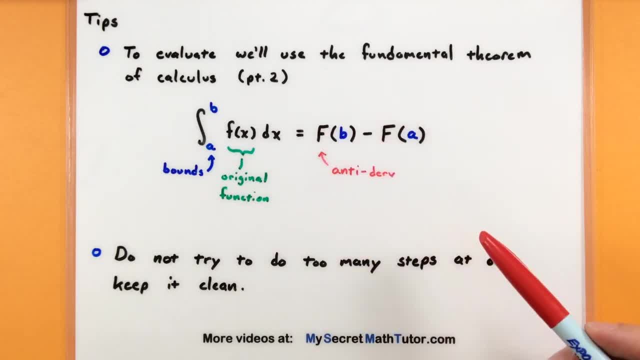 of calculus, what some people would call the FTC part two, And the way that works is: you're going to take a look at your integral and you're going to find the antiderivative of this original inside function And then you're going to plug in the top and bottom bounds and subtract the two. 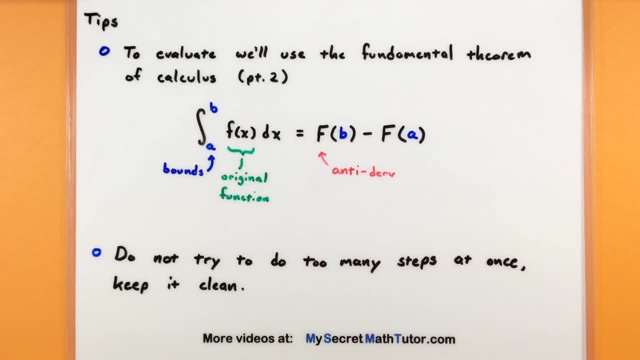 Now the tough part about this is that you really just want to keep things nice and clean while you're going through these different steps. In other words, do not try and do too many steps at once and definitely keep it clean. It's really just a lot of bookkeeping And, of course, trying. 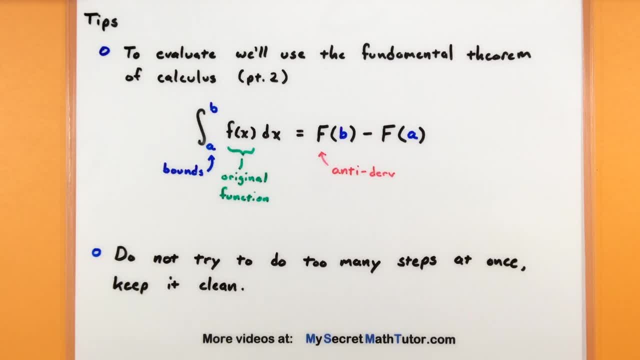 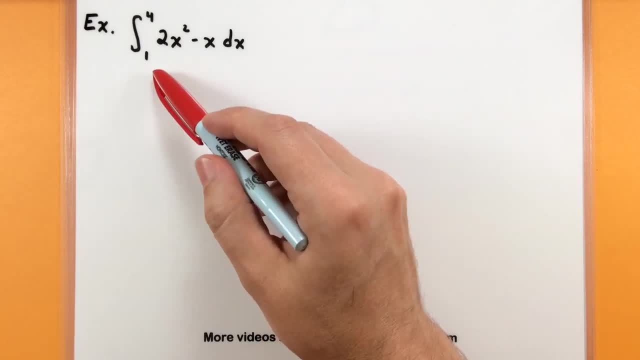 to find that antiderivative so that you can get to that next step. Alright, let's go ahead and look at the example. See exactly what I'm talking about. So in this first one I'm dealing with the integral from one to four of two x squared minus x, And then the first step you really just want. 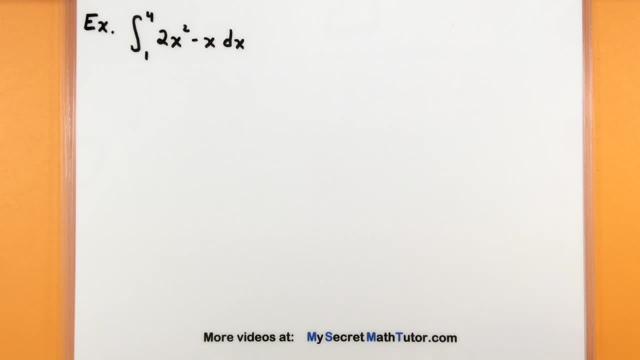 to worry about finding the integral of x squared minus x. And then, the first step: you really just want to worry about finding the integral of x squared minus x. And then, the first step: you really just want to worry about finding that antiderivative. Yes, we'll eventually plug in the bounds and do all that fun stuff, But you 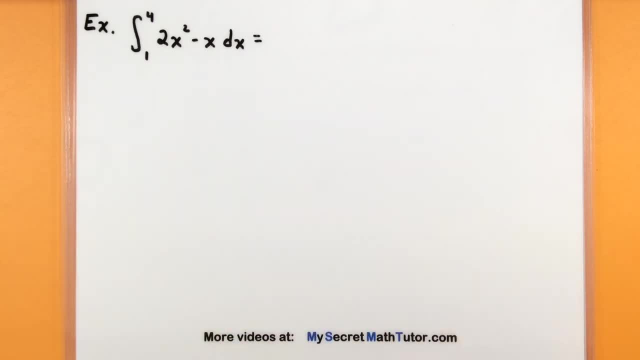 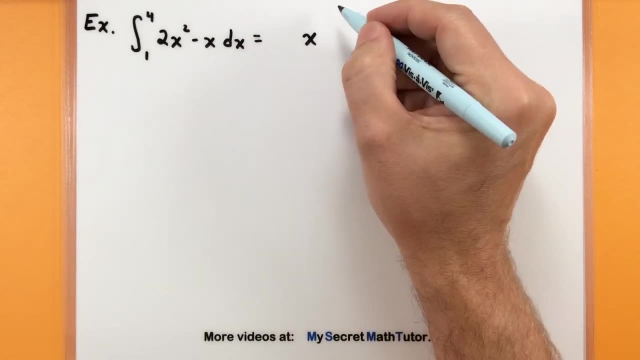 know, don't worry about that for now. Just look at the function and see if you can find its antiderivative In this particular one. I'm going to use a power rule, So we'll add one to the power. In this case, it goes from two to three And we'll divide by that new power. 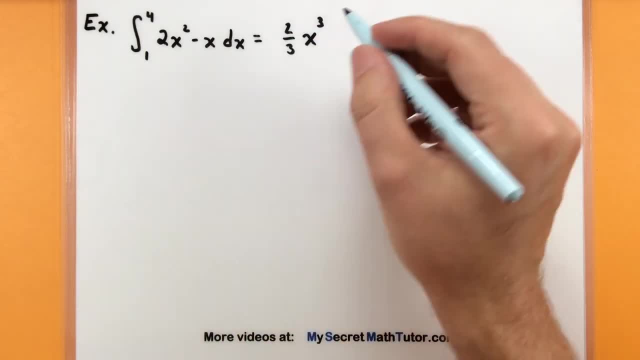 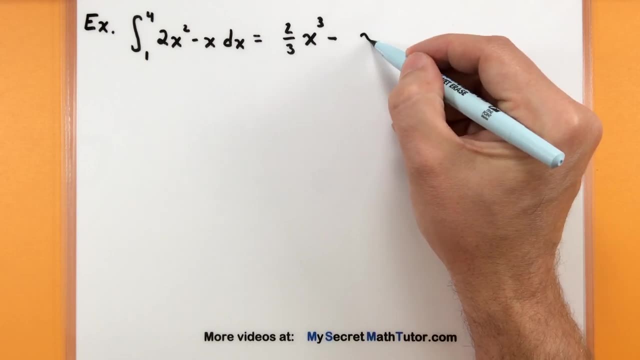 So two is going to be divided by three- See next part. here, since it's being subtracted, I can just find its antiderivative And we'll do the same thing. We'll add one to the power, I'll turn it into a two and we'll divide by that new power. 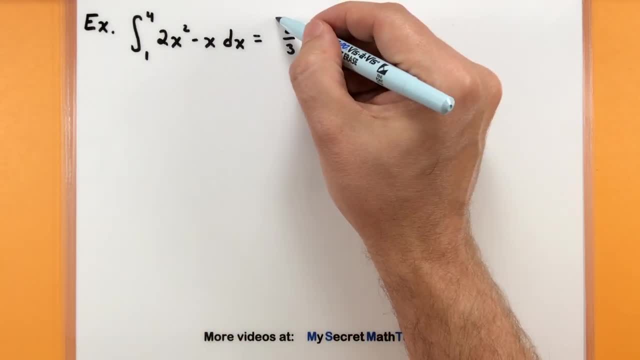 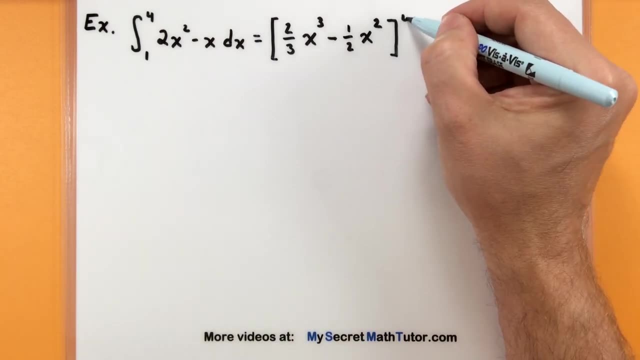 So here in this first step, I'm only finding an antiderivative. The way I want to remember that I still need to plug in some bounds into this is: I like to put in a pair of square brackets and then put in my bounds right off to the side. 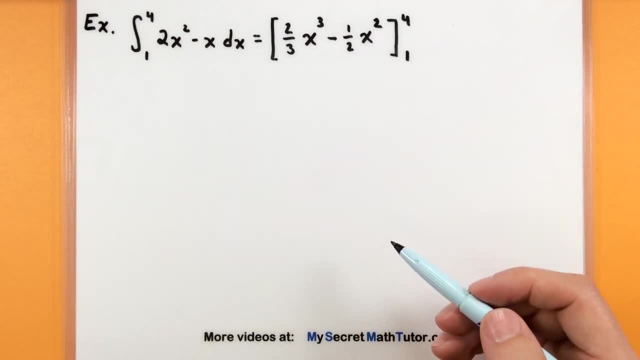 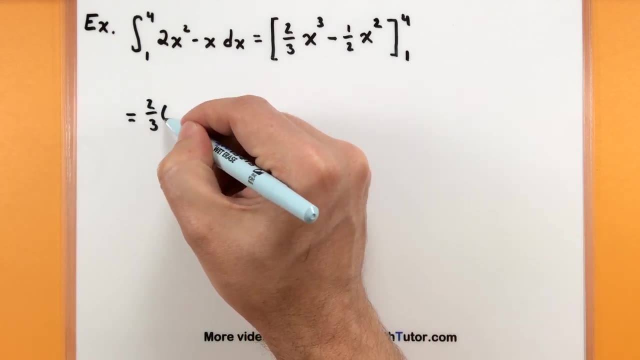 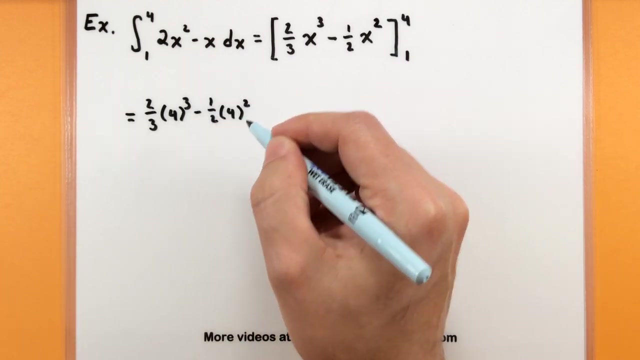 That tells me: yes, I found the antiderivative. Now it's time to evaluate this. Alright, so let's do that. So you want to write your expression for the antiderivative here, Starting with the top bound plugged in, And then we'll go ahead and plug in the bottom bound. So let's see, that's all good. 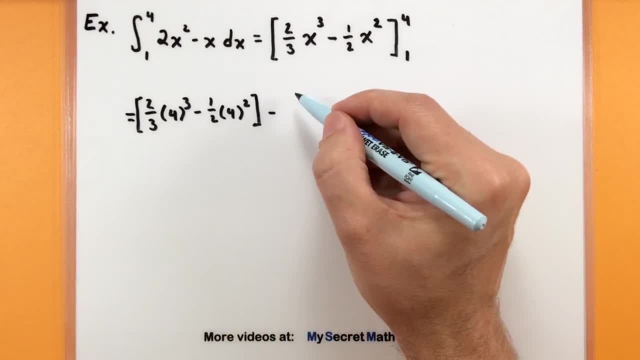 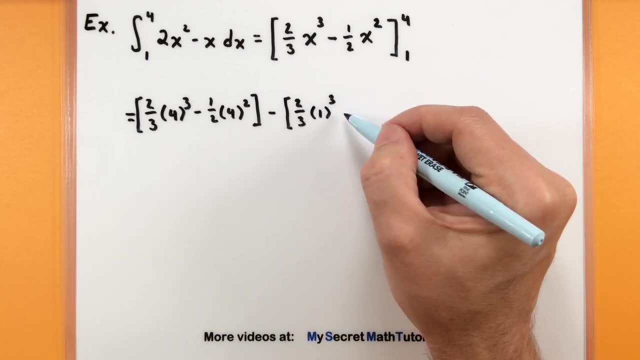 I'm going to leave this in a square bracket to make sure that I keep that all combined together, And then let's go ahead and plug in the bottom bound. Now, the important part about having this in brackets here is we want to subtract this entire. 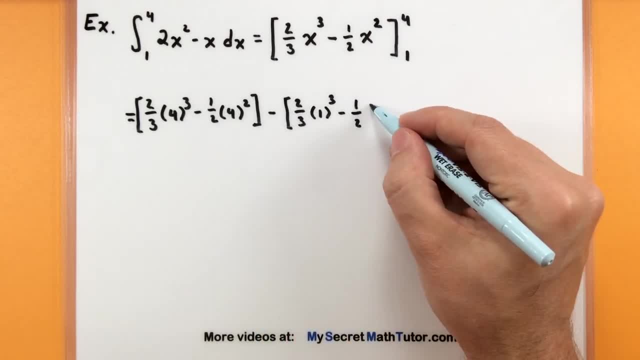 second piece, If I didn't put in some grouping symbols here of some sort. it's often a common mistake to do that. So let's go ahead and plug in the bottom bound, And then we'll go ahead and plug in this inside the middle box, And then will let's. let's see what this does. 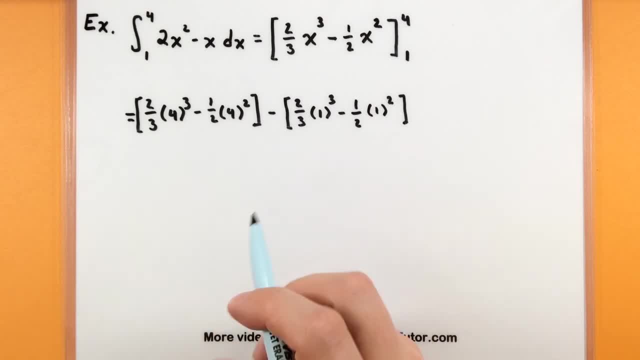 Alright, let's go ahead and plug in the bottom out of our insgesamt hardscore here, because we'll get something back that's running really pretty fast too. So let's go ahead and plug in this int, ent, pastor- almost The term int shows. take us zed by t and it probably doesn't spend as much power. 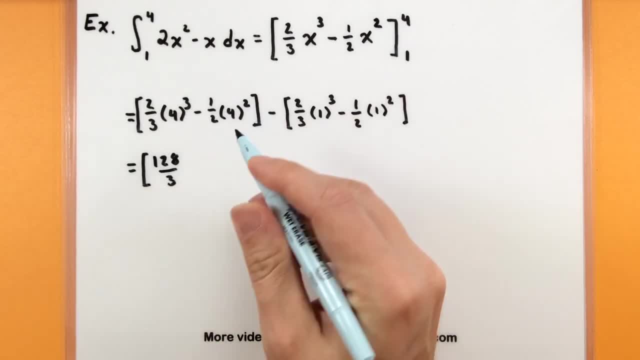 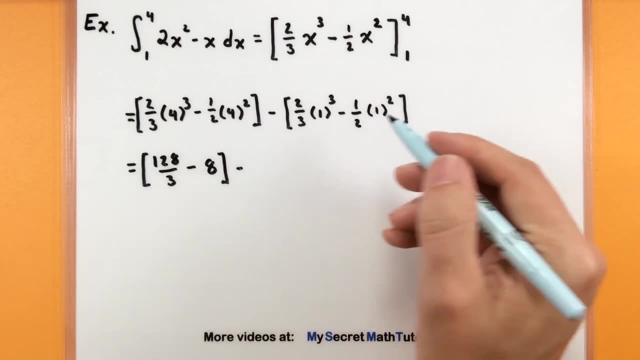 but this supposed to mean that each of these objices are going to be having this thing. And then what that means? oh, okay, but it depends. Let's see off to the other side here. One cubed is just one, so that'll be one times two-thirds. 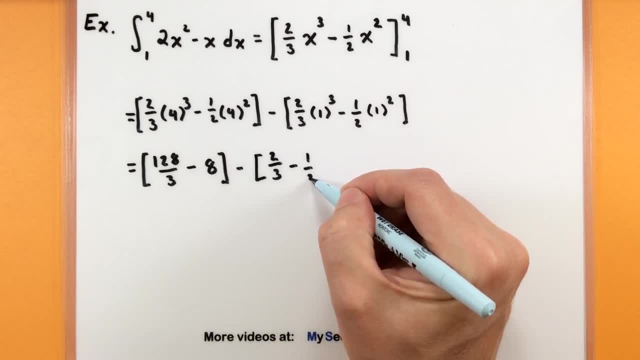 There's the two-thirds, And one squared is one, so there's our one-half. So things are looking fine. I'm definitely keeping those grouping symbols as much as I can, you know, simplifying, But eventually we will go ahead and distribute into the second grouping symbol. 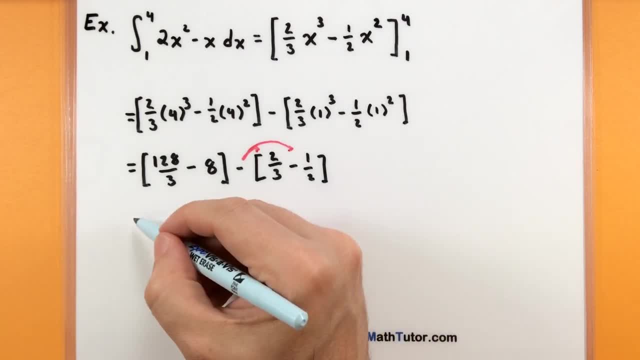 That way, we can actually start combining even more things. All right, so let's see. What does that give us? Well, this will still be 128 all over, 3 minus 8. And then we'll have a minus two-thirds. 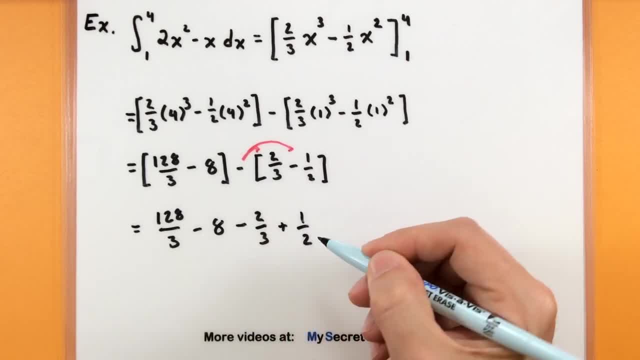 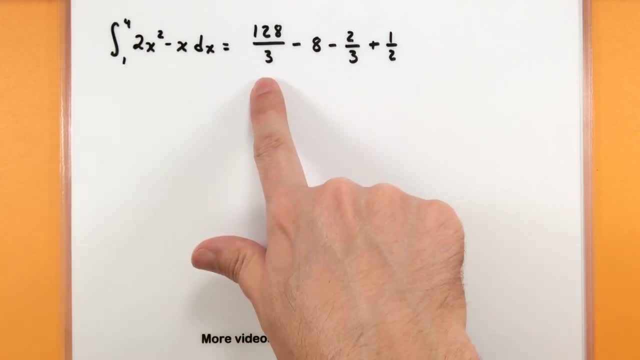 Then minus, minus will give us a plus one-half. All right, so as we're going through this algebra, we are making progress. Essentially, we've taken our integral and just turned it into these numbers And again we just have a little bit more algebra. to go ahead and take it farther. 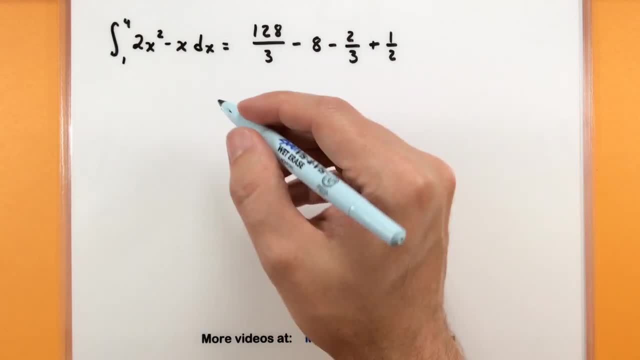 128,. if I subtract the two, since these both have the same denominator, that will give me a 128.. 126 over 3.. And then I still have this minus 8 and a plus one-half. All right, that's not looking too bad. 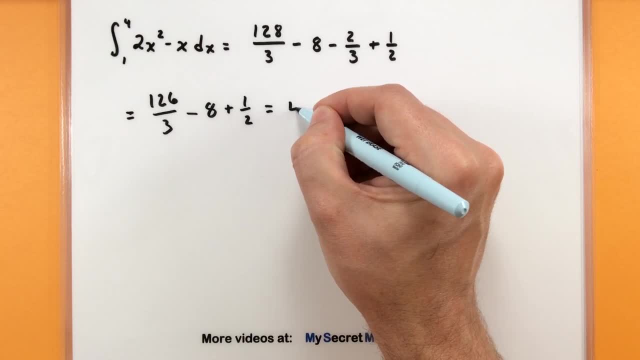 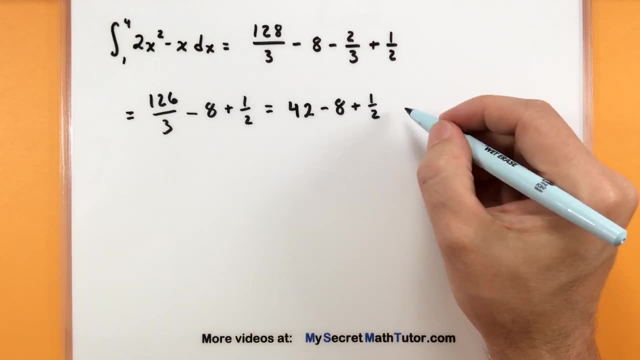 Let's see 126 divided by 3, that simplifies nicely. That turns into a 42. So now I have 42 minus 8. We can simplify that into a 34.. So I'm really looking at 34 plus one-half. 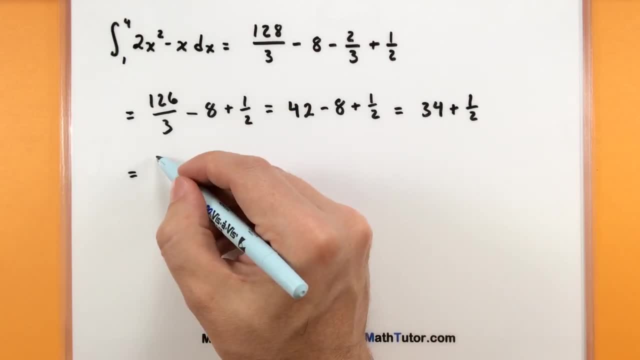 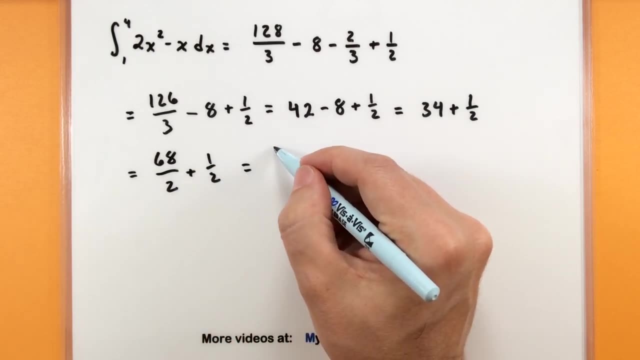 If we want we can. We can go ahead and combine those by finding a common denominator. So that'd be a 68 over 2 plus one-half, So we can call this a 69 over half. So there's really a couple of ways you could write your answer. 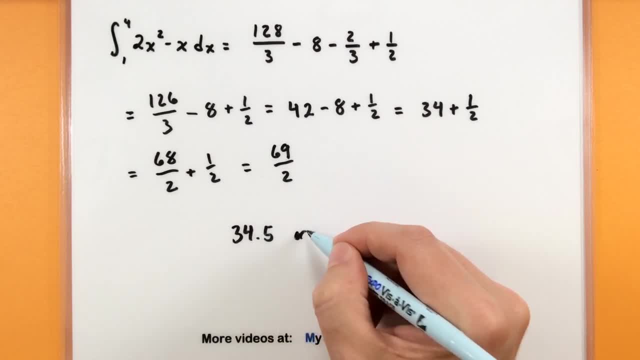 You could leave it as the 34 and a half, Or if you want to write it as a fraction, you could write it as the 69 and a half. Either way, that would give us the value of our definite integral. Now, just to show you the importance of finding that antiderivative and an excuse to do just one-half: 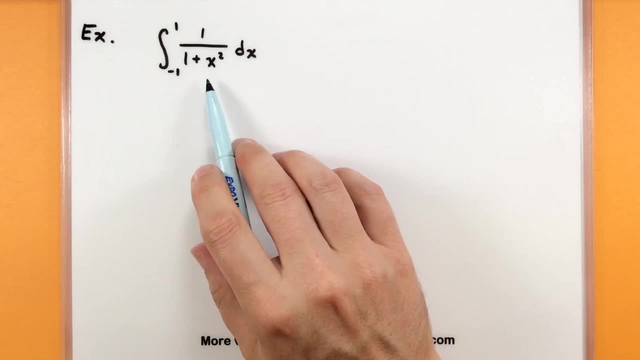 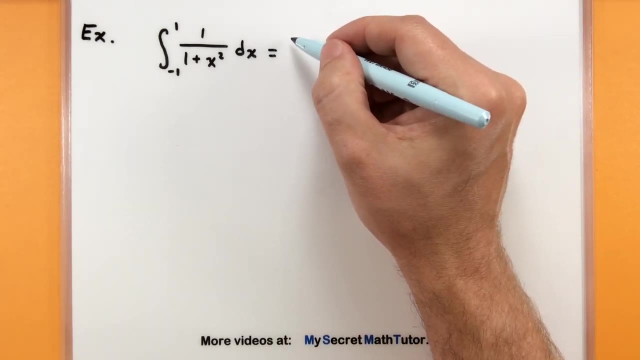 just one more example. we'll do this guy right here. So we look at this integral and you want to think carefully about your antiderivatives for the inside In this particular one. even though it may not seem like a common one, you want to remember it. 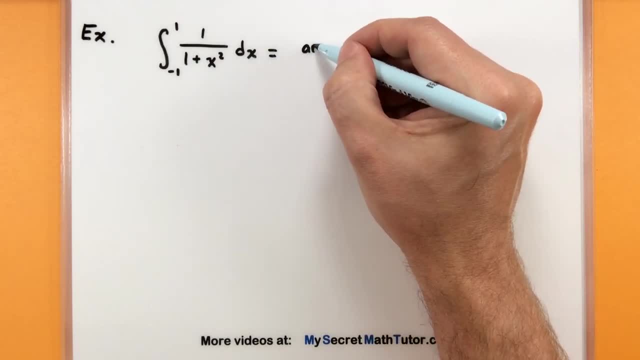 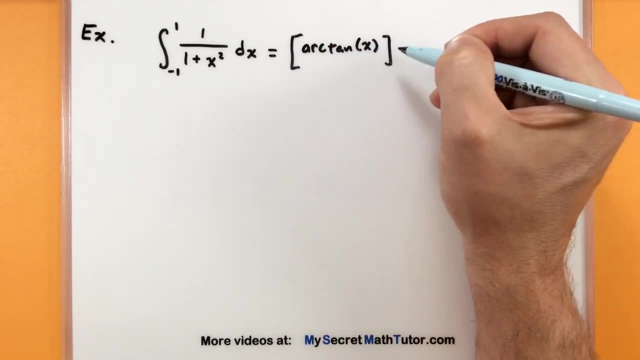 The antiderivative of 1 over 1 plus x, squared is arctangent. This seems to be a very common one that teachers like to throw on exams or whatnot when finding antiderivatives. Of course you got to know your inverse trigonometric functions to be able to do this. 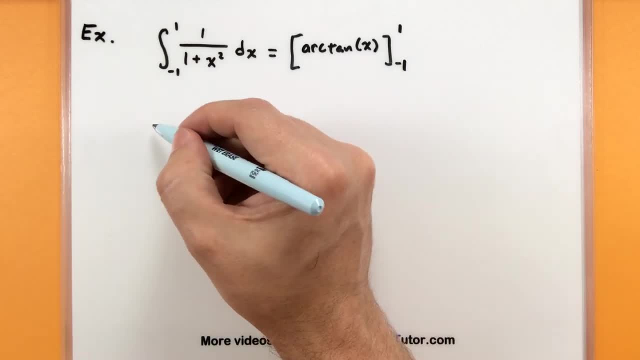 All right, So we have our antiderivative. That's just the first step. Now let's go ahead and plug in our bounds. So, even though it's kind of a strange-looking function, we're just going to evaluate it at the top bound minus. 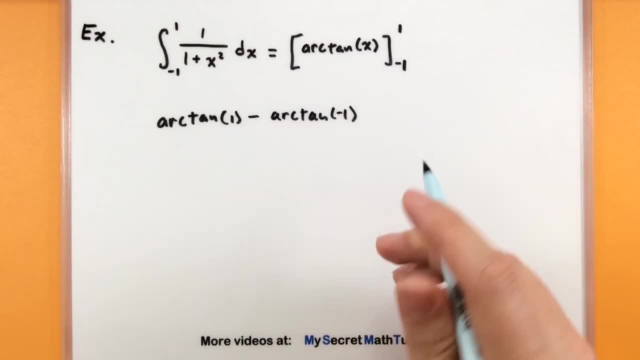 and then evaluate it at the bottom bound. So nothing too crazy. I just have to figure out what is the value of arctangent of 1 and negative 1.. These aren't too bad. Arctangent of 1 is just a pi over 4, minus, and arctangent of negative 1, this will be a negative pi over 4.. 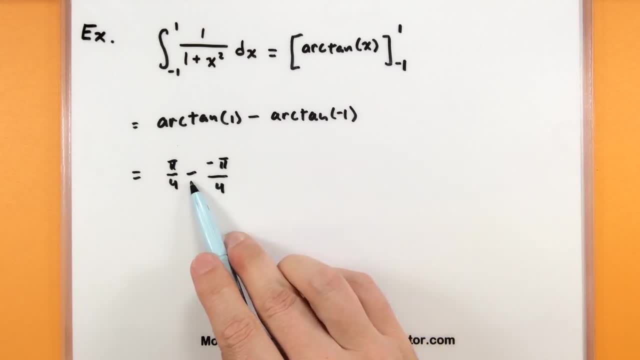 So here again, I'm being really careful What to do with my negative signs. This negative sign comes from subtracting both my antiderivatives. This negative sign comes from evaluating this arctangent of negative 1.. All right, So pi over 4, minus and minus will give us a plus. 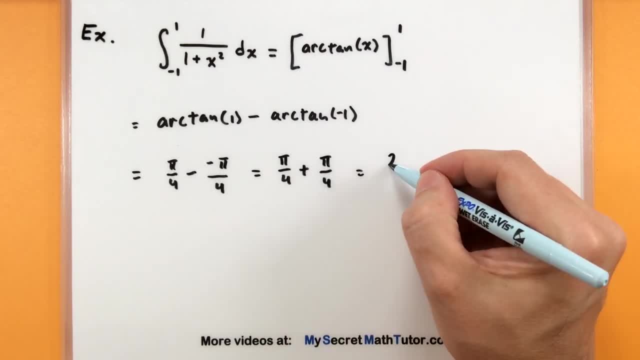 So we just have 1 fourth pi plus another fourth pi. We have a total of 2 fourths pi, or 2 pi over 4, no matter what you want to call it. So this gives us just pi over 2 when we reduce it. 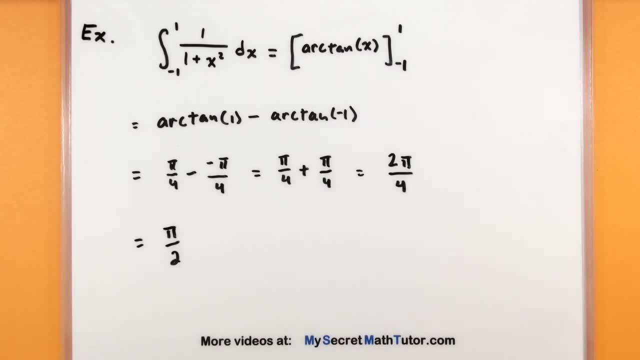 And there's our answer. So you can see doing definite integrals. It's not that hard, It's not so bad. You really just have to find the antiderivative and then go ahead and plug in your bounds, starting with the top and the bottom. subtract the 2..